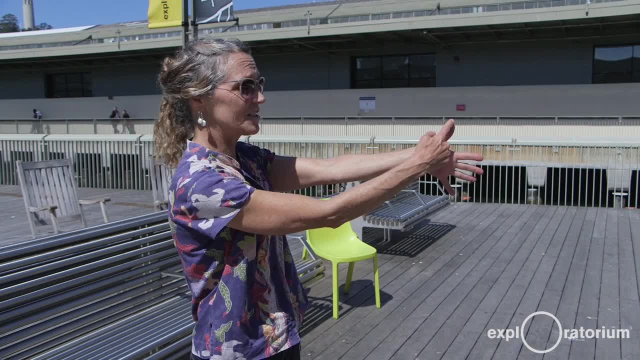 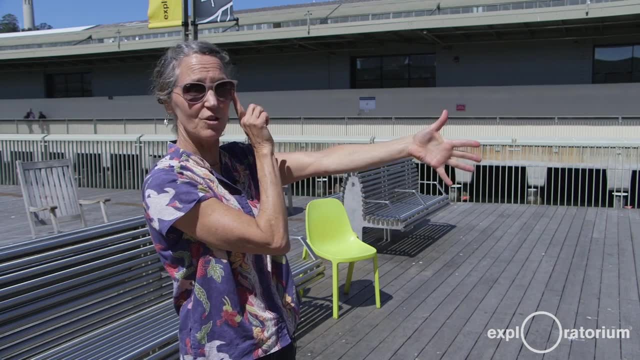 this because I'm using a simple ratio, The ratio of the distance from my thumb to my little finger when my hand is outstretched, and using that as a height, the distance to my eye, This what I'm calling a height now, from the tip of my thumb to my thumb. 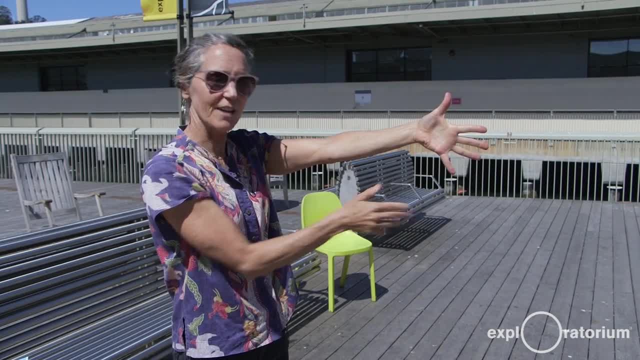 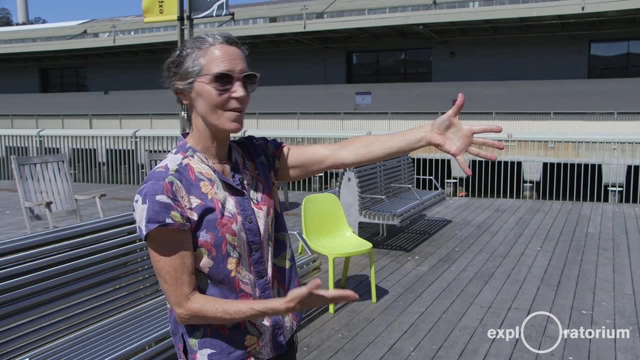 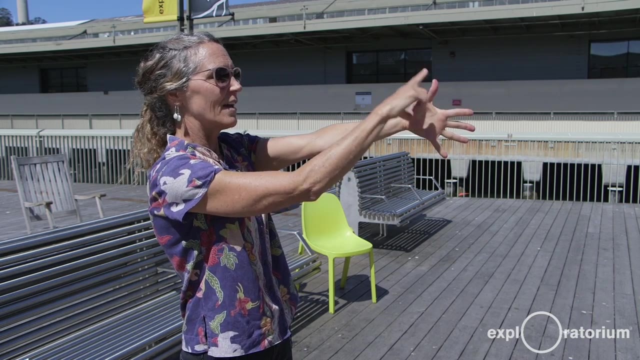 to my little finger when my hand is outstretched has a name. in some Spanish speaking cultures It's called una cuarta, and people use it as a non-standard measuring tool. I need to know my ratio of una cuarta, or the height of my outstretched hand to my eye, And so I'm going. 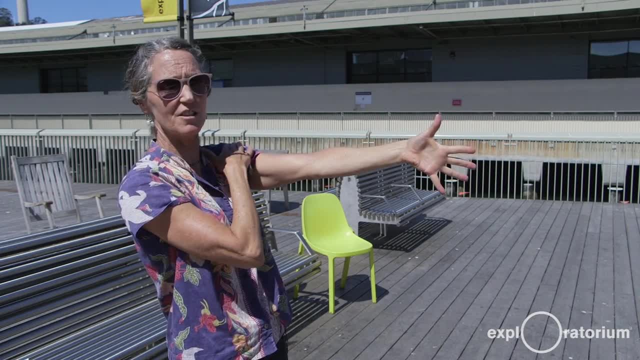 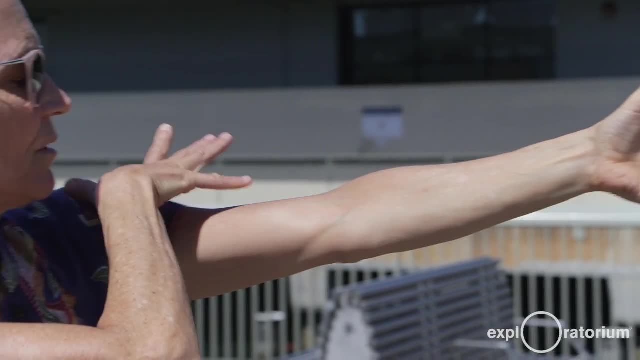 to measure the length of my arm, which is pretty much the distance to my eye using my outstretched hand. There's one, two, three, four, five, six, seven, eight, nine, ten, 11,, 12,, 13,, 14,, 15,, 16,, 17,, 18,, 19,, 20,, 21,, 22, 23.. When I get to my shoulder I'm pretty. 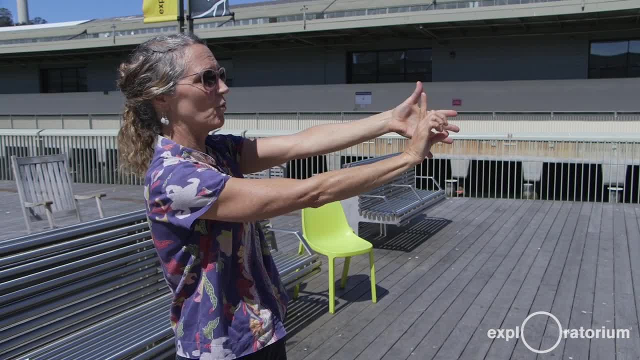 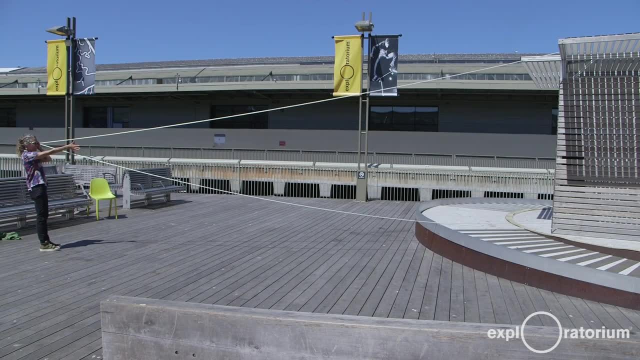 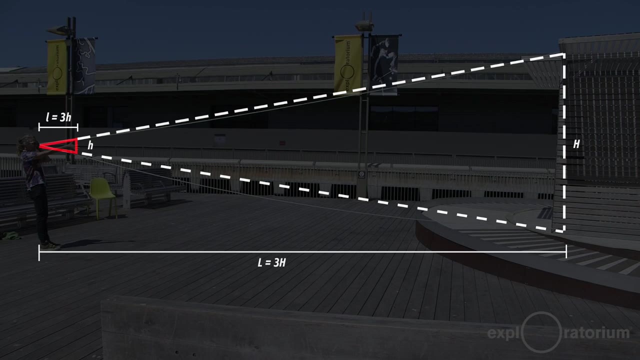 much, even with my eye, And so I have shown you that there is a one to three ratio. When the string is outstretched, you can see that I have two similar triangles: One that's formed by the side of the building and going back to my eye, and the embedded similar triangle. 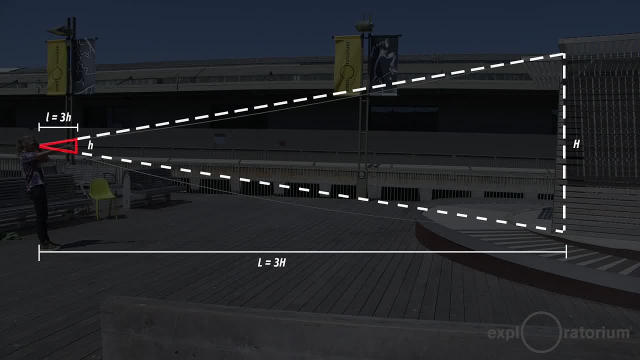 formed by my cuarta. going back to my eye, Because these are similar triangles, that one to three is equal to one, And so I'm going to measure the length of my arm, which is a three ratio that we measured with my cuarta, and the length of my arm is equal to the ratio. 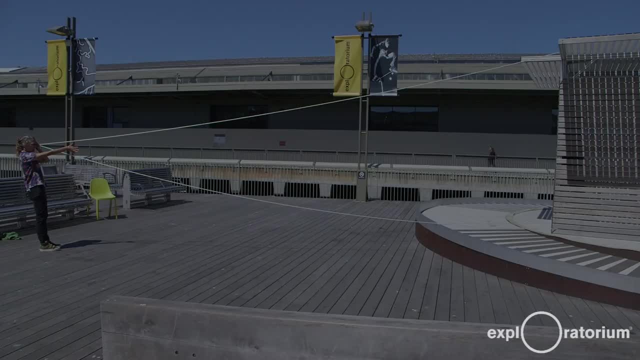 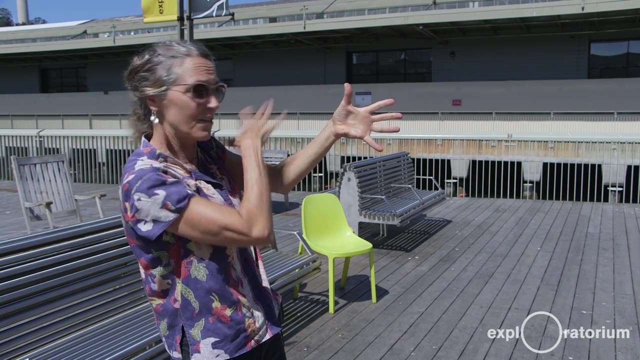 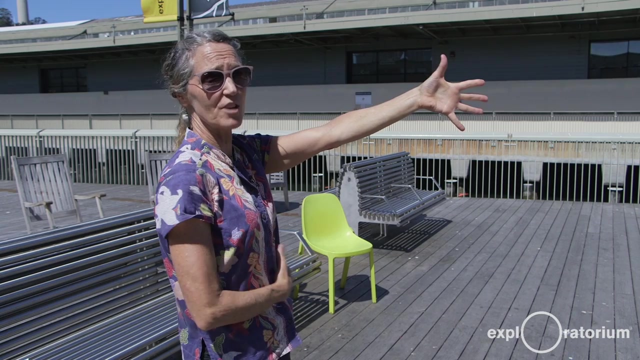 of the height of my building and my distance to it. What's important in making this measurement is that my elbow remains straight. If I bend my elbow, this is not three distances away from my eye any longer. Elbow has to remain straight and I'm going to face the object. 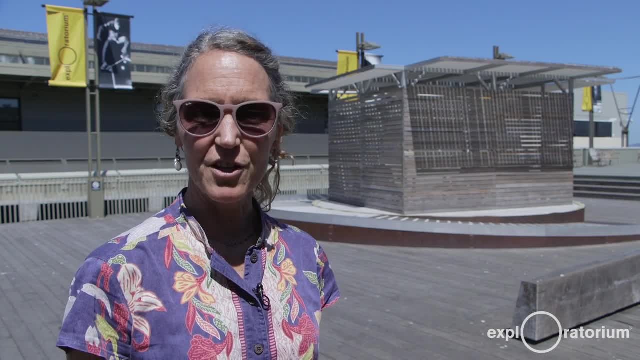 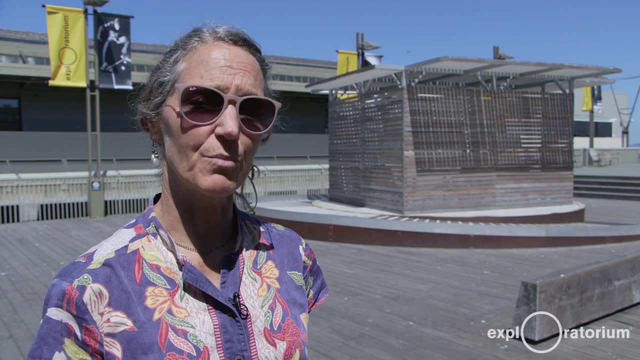 that I'm measuring When I'm solving for an unknown in a proportion. all I need to know is three of the measurements. I know: my one to three ratio of my cuarta to the length of my arm and to measure the height of that building. all I need to know is my 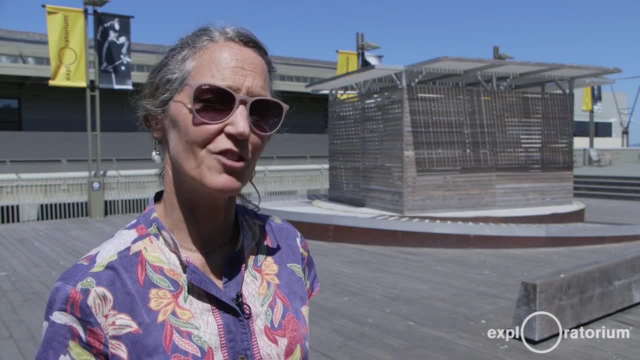 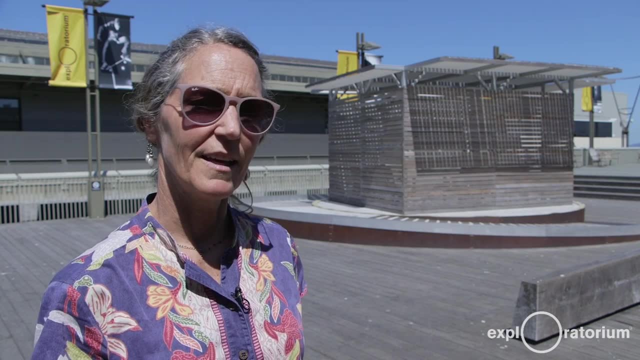 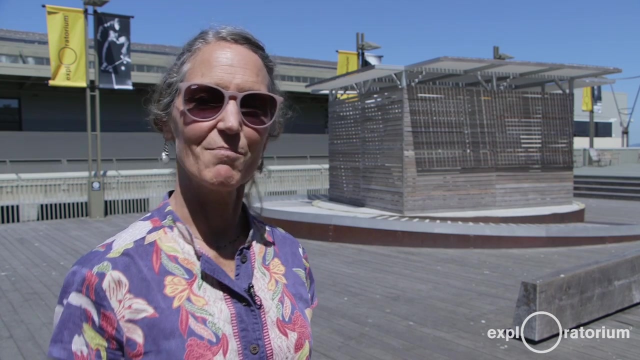 distance to it. I measured the distance to the building just now and it was 7.5 meters. If it's also a one to three ratio, where the height of the building is one third of the distance to it, that means the height of that building is 2.5 meters. I can use that to measure the height of the building.